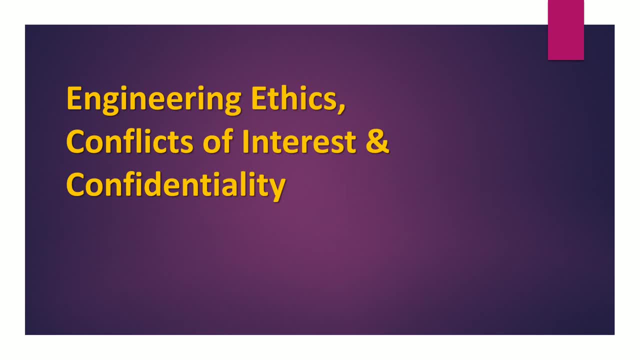 Today we are discussing some other important topics, like what is actually the engineering ethics and what are all the different conflicts that will occur in the construction company and in the profession, and what is confidentiality. These are all the things we will discuss today and we will come to an end of third module. 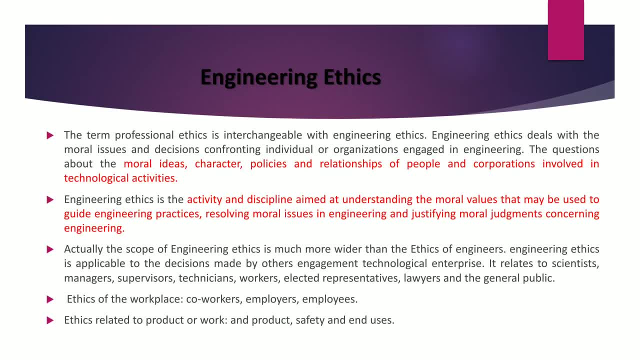 So we will begin with the engineering ethics. So the term professional ethics is interchangeable with engineering ethics. Engineering ethics deals with the moral issues and decisions confronting individuals or organizations engaged in engineering: The question about the moral ideas, characters, policies, relationships of people and corporations involved in the technological activities. 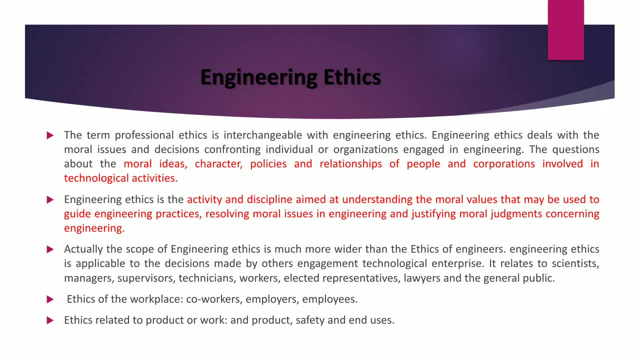 So engineering ethics is the activity and the discipline aimed at understanding the moral values that may be used to guide engineering practices, resolving moral issues in engineering And justifying moral judgements concerning the engineering. Actually, the scope of engineering ethics is much more wider than the ethics of engineers. 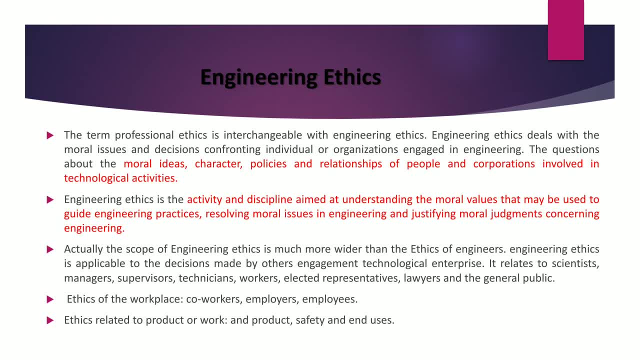 Engineering ethics is applicable to the decisions made by other engagement technological enterprises. It relates to scientist, manager, supervisor, technical workers, elected representatives, lawyers and general public. So ethics of the workplace are concerned with coworkers, employees and employees, co-workers, employees and employers, whereas ethics related to the product or work depends upon the. 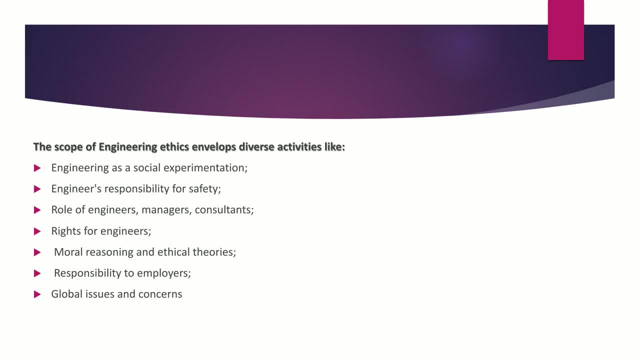 product safety and end users. so what are the different scopes of engineering? takes up engineering as a social experimentation, engineers, responsibility for safety, role of engineers, managers, consultants, rights of engineers and moral reasoning and ethical theories reasonably to employ, responsibility to employers and global issues and concerns. so what are the? 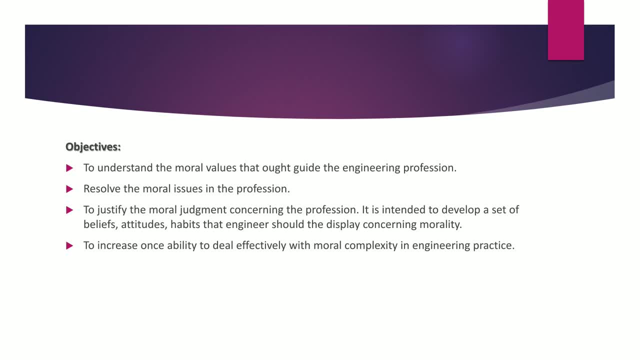 different objectives: to understand the moral values that out guide the engineering profession, resolve the moral issues in the profession. to justify the moral judgment concerning the profession. it is intended to develop a set of benefits, attitudes, habits that engineers should be display concerning morality, and to increase one's ability to deal effectively with the 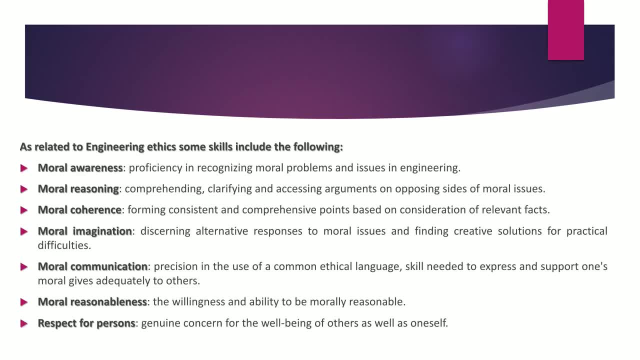 home moral complexity in engineering practice. so, as related to engineering ethics, some skills should be implemented. those are more: 11: that is proficiency in recognizing moral problems and issues in engineering and moral reasoning. that is comprehending, clarifying and accessing arguments on opposing sides of the moral issues and moral coherence forming. 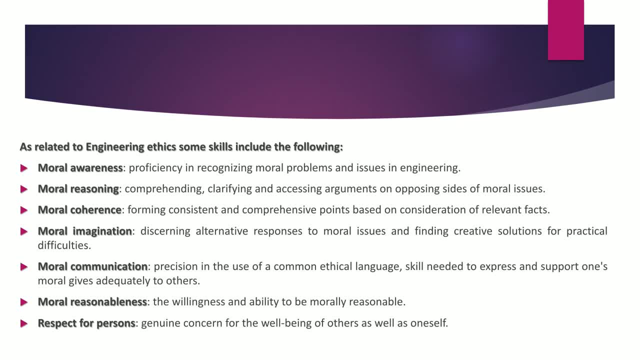 consistent and comprehensive points based on considerations of relevant facts and moral imagination. that is, describing alternative responses to moral issues and finding creative solutions for practical difficulties, whereas moral communication is precision in the use of common ethical language. skills need to express the support once moral gives adequate to others. 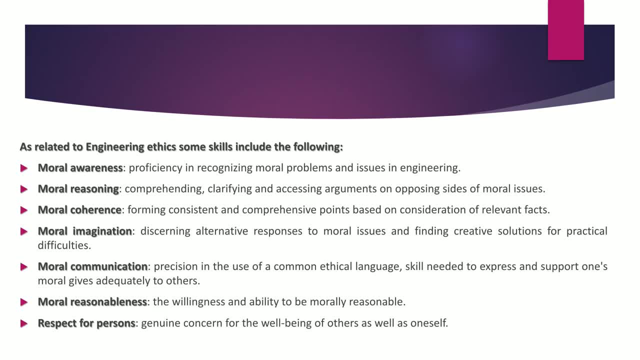 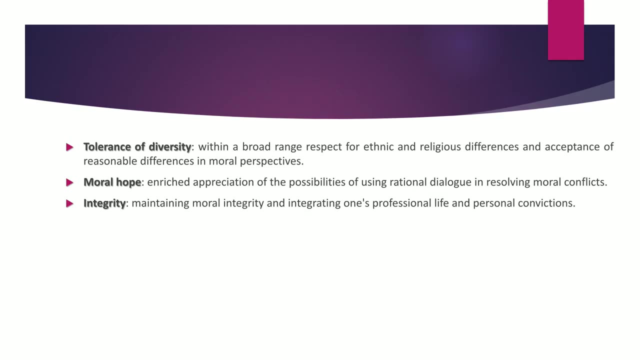 next, moral. moral reasonableness, that is, the willingness and the ability to be morally reasonable and respect for persons, genuine concerns for the well-being of others as well as oneself, and tolerance of diversity. that is, within a broad range, respect for ethnic and religious differences and acceptance of reasonable differences in moral perspectives and moral hope. 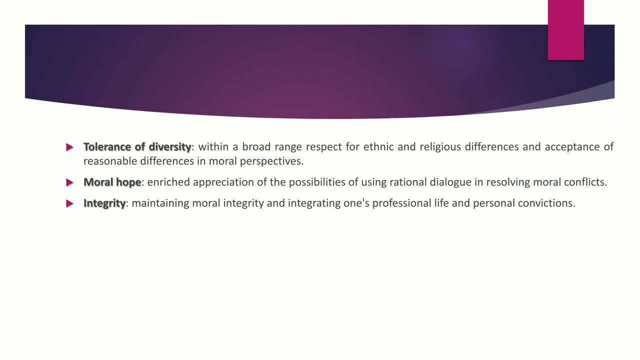 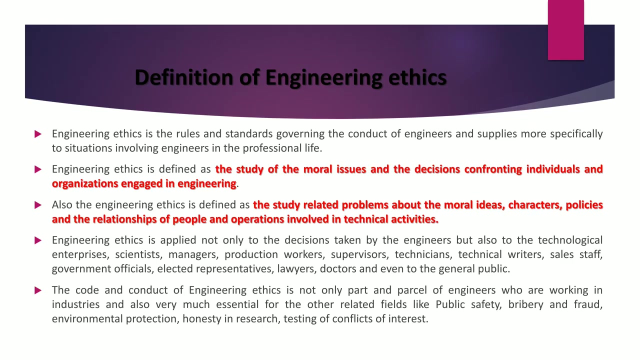 that is, the enriched appreciation of the possibilities of using rational dialogue in resolving moral conflicts and integrity, maintaining moral integrity and integrating one's professional life and personal convictions. these are some skills to be implemented in engineering field as a. as i mentioned, it's a based on engineering ethics. 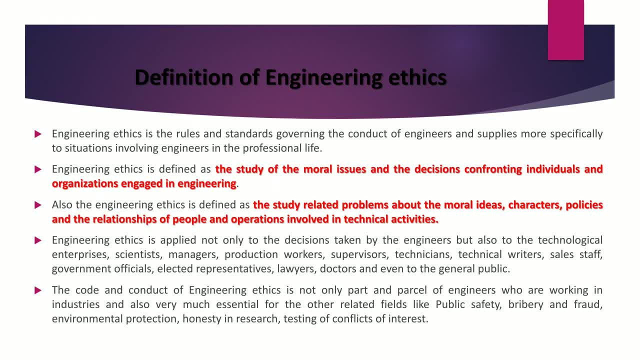 next, what is the definition of engineering ethics? it is the rules and standards governing the conduct of engineers and suppliers, more specifically, to situations involving in engineering in the professional life. it is defined as the study of the moral issues and decisions confronting individuals and organizations engaged in engineering, and also it can be defined as the 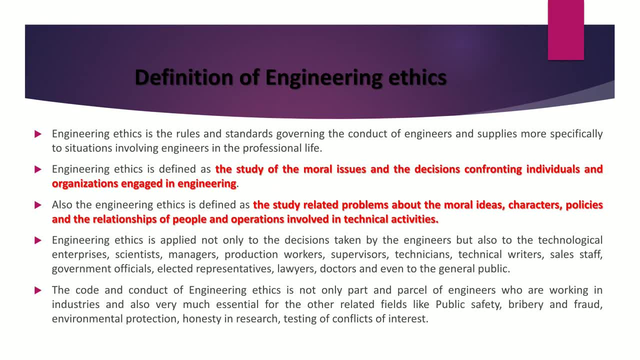 speed theory, theory of the public study and and approach algorithmic problems about the moral ideas, characters, policies and the relationships of the people and operations involved in technical activities. it is applied not only to the decisions taken by the engineers but also technological enterprises. scientists, managers yesterday could sell stuff, government officials, elected representatives, lawyers, doctors, and given to the general public. the code and conduct of engineering ethics is not only part and parson ethics regulation, including Suz GA, many Barbados concecases, hydrophobia, Asians, folio rights. 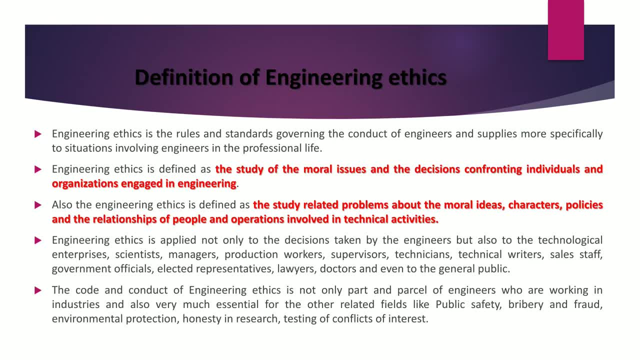 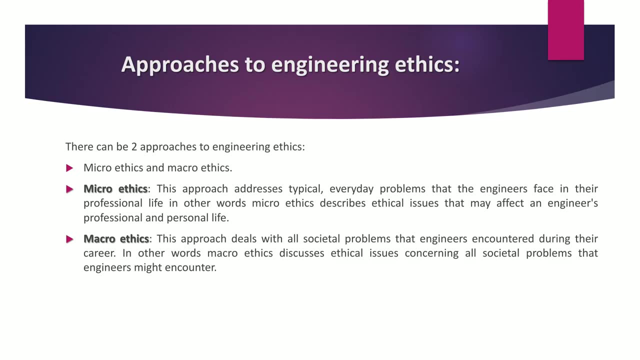 of engineers who are working in the industries and also very much essential for the other related fields like public safety, bribery and fraud, environmental protection, honest in research, testing of conflicts of interest, etc. so which are all the different approaches to engineering? it is mainly, basically, there are two approaches: decision: micro ethics and macro ethics. so what is micro ethics? 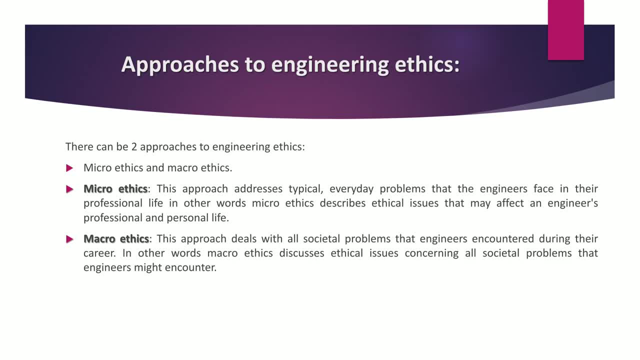 this approach addresses typical everyday problem that the engineer face in their professional life. in other words, micro ethics describes ethical issues that may affect an engineer's professional and personal life, whereas macro it deals with the social, societal problems that engineers encode during their career. in other words, micro ethics discusses ethical issues concerning all societal 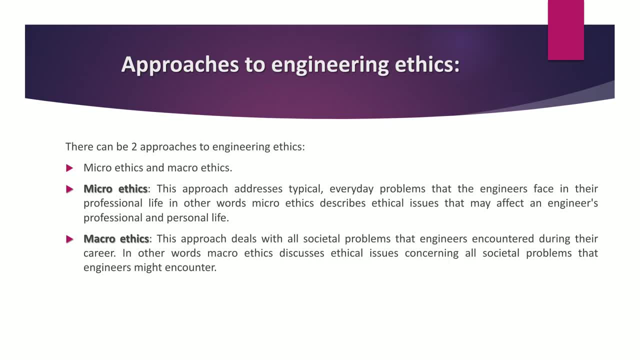 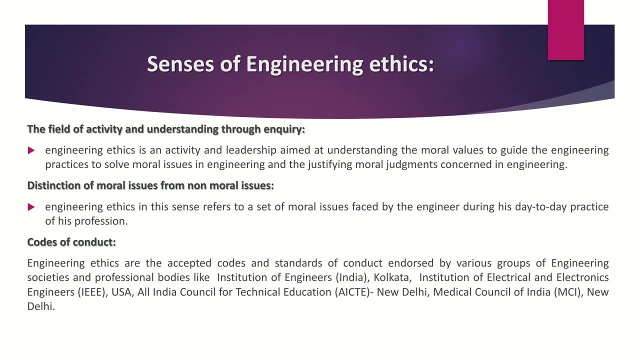 problems that engineers might incur. micro ethics is a personal relations with the engineer, whereas macro is related for the society, societal problems. so which are the different senses of engineering ethics? engineering ethics is an activity and leadership aimed at to understand the moral values, to guide the engineering practices, to solve moral issues in 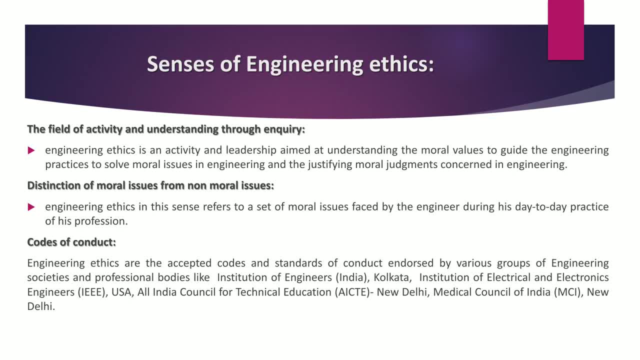 engineering and the justifying moral judgment concern in engineering. so first one is a distinction of moral issues for non moral issues. that is, engineering ethics in this sense refers to a set of moral issues faced by engineer during his day-to-day practice or his profession. second one is codes of conduct. engineering ethics are accepted. 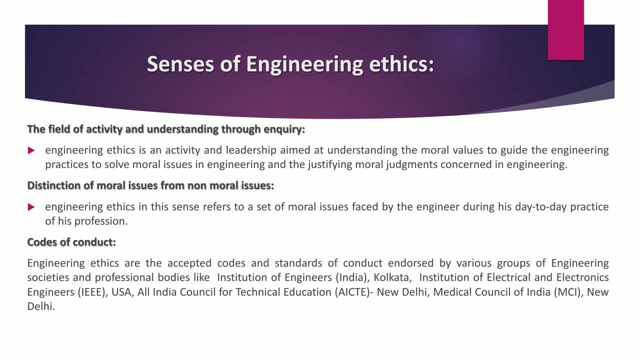 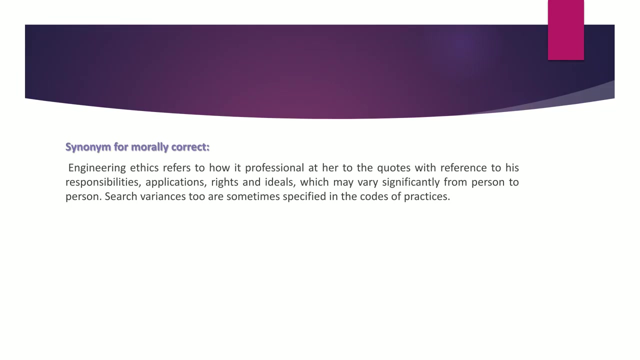 codes and standards of conduct endorsed by various groups of engineering societies and other professional bodies, like Institute of engineers and instead of electrical and electronics engineers and all India Council for Technical Education and Medical Council of India, etc. next last one is synonym for morally correct, that's engineering ethics refers to how it professional and 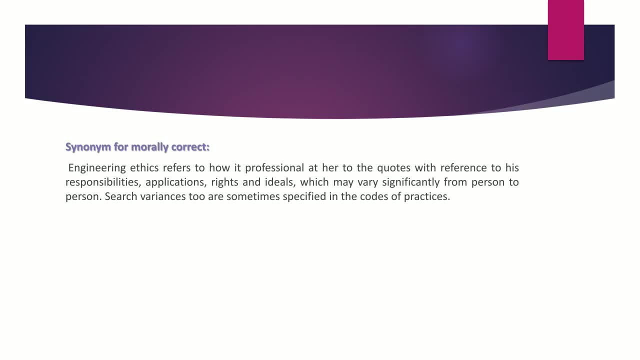 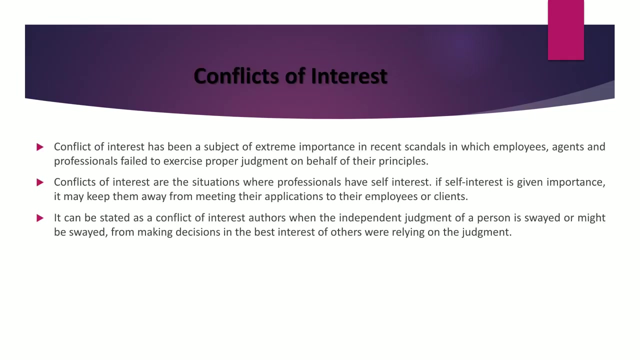 professional involvement at her it to the courts with reference to his responsibility, responsibilities, applications, rights and ideals, which may vary significantly from person to person. such way, variances to are sometimes specified in the course of practices. so conflicts of interest. next comes, what is actually the conflict of interest? 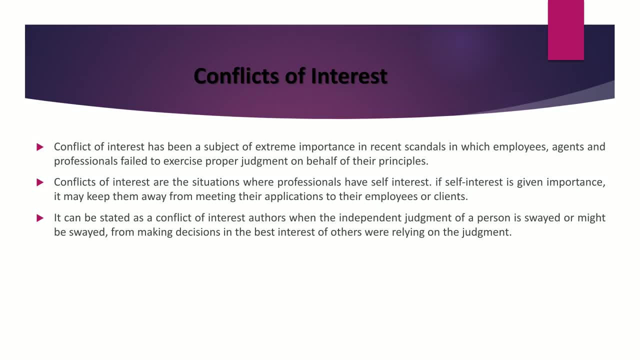 It has been a subject of extreme importance in recent scandals in which employees, agents and professionals fail to exercise proper judgment on behalf of their principals. These are the situations where professionals have self-interest. If self-interest is given importance, it may keep them away from meeting their application. 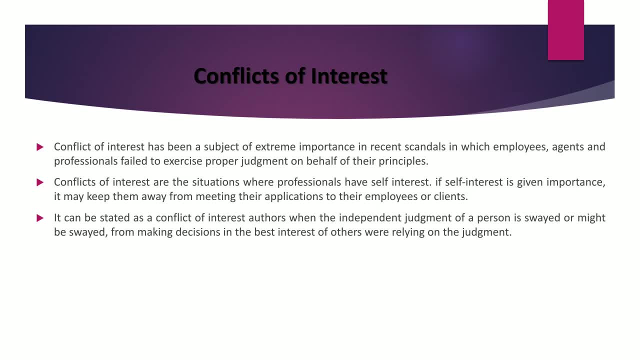 to their employees or clients. So it can be stated as a conflict of interest. authors, when the independent judgment of a person is swayed or might be swayed, from making decisions in the best interest of others were relying on the judgment. So which are the different types of conflicts of interest? 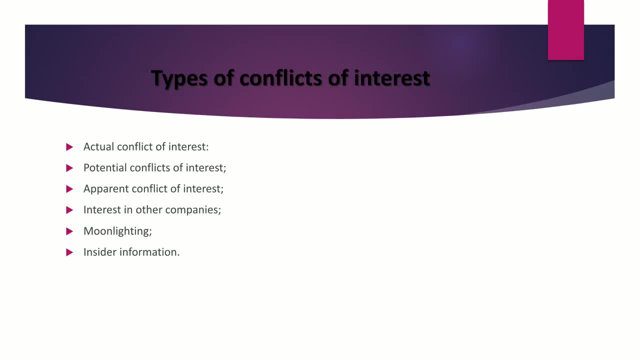 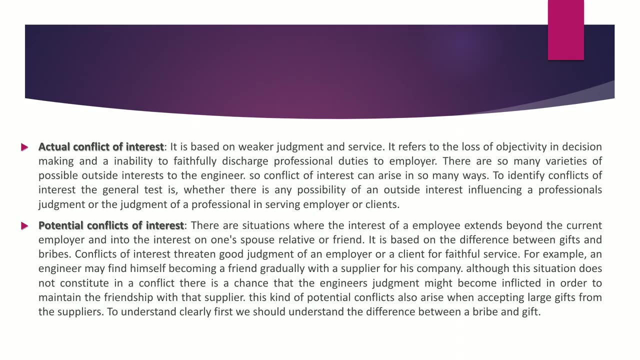 That is actual conflict of interest, potential conflict of interest, apparent conflict of interest, interest in other companies and moonlighting and insider information. What is actual conflict? It is based on weaker judgment and surveys. It refers to the loss of objectivity in decisions. 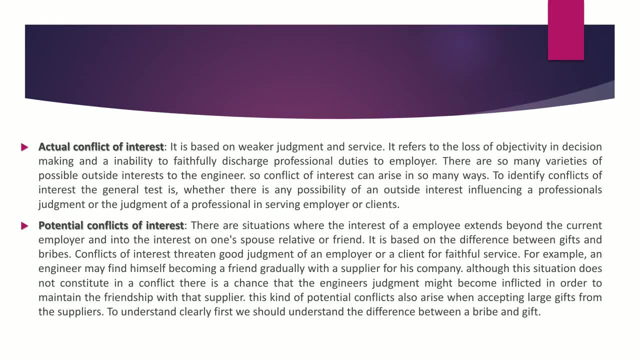 It refers to the loss of ability to make decisions and the inability to faithfully discharge professional duties to the employer. There are so many varieties of possible outside interest to the engineer, So conflict of interest can arise in so many ways. To identify conflicts of interest, the general test is whether there is any possibility of 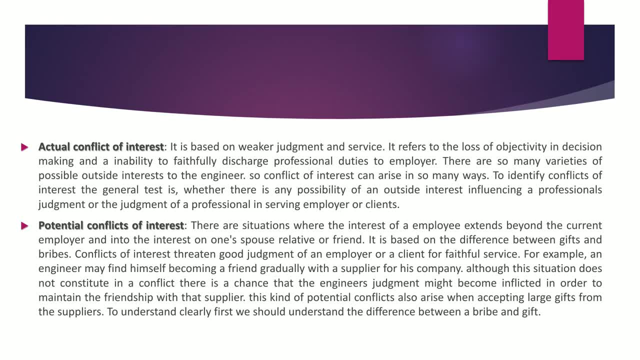 an outside interest influencing a professional judgment or the judgment of a professional is serving employers or clients. Second one is potential conflicts of interest. The second one is potential conflicts of interest. The second one is potential conflicts of interest. There are situations where the interest of employees extend beyond the current employer. 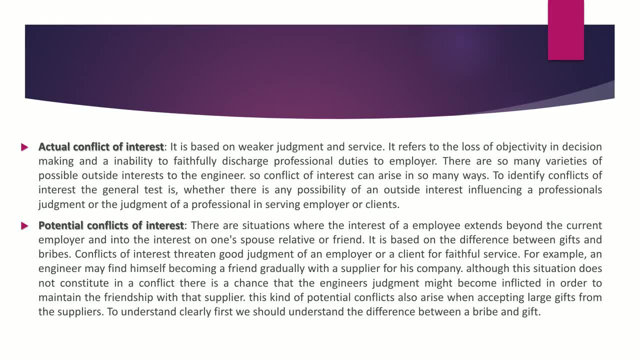 and into the interest of one's spouse, relative or friend. So it is based on difference between the gifts and bribes. So conflicts of interest have threatened good judgment of an employer or a client for faithful service. For example, an engineer may find himself becoming a friend gradually with the supplier. 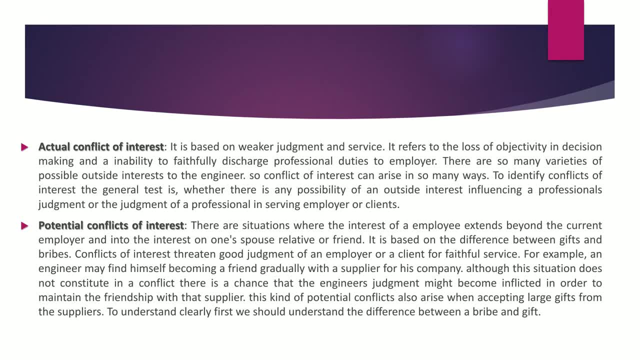 for his company. Although this situation does not constitute in conflict, There is a chance that the engineer's judgment might become inflicted in order to maintain the friendship with that supplier. This kind of potential conflicts also arise when accepting large gifts from the supplier. So to understand clearly, first we should understand the difference between the bribe. 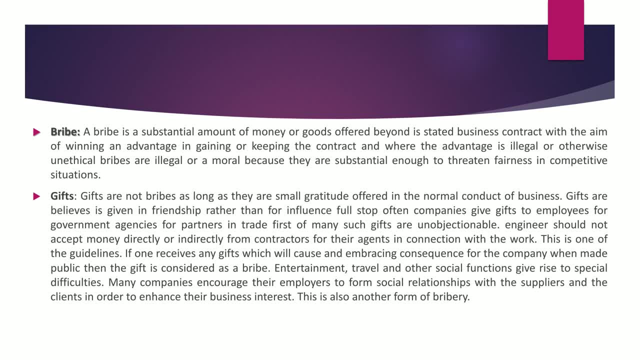 and gift. So bribe is nothing but a substantial amount of money or goods offered beyond its stated business contract with the aim of winning an advantage. So this is the difference between bribes and gifts. In bribes, the only upfront and indirect benefits of offer will be the 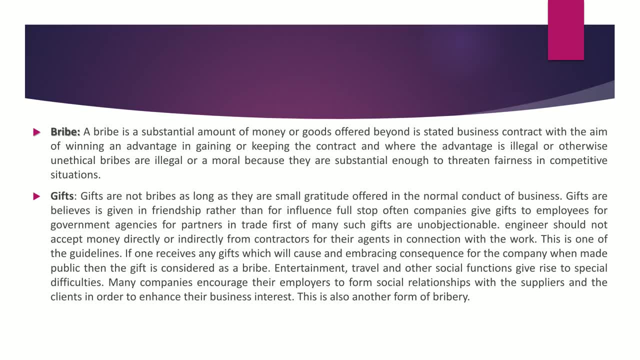 Often companies give gifts to employees, for government agencies, for partnerships in trade first, and many such gifts are unobjectionable. Engineers should not accept money directly or indirectly from contractors for their agents in connection with the work. This is one of the guidelines. 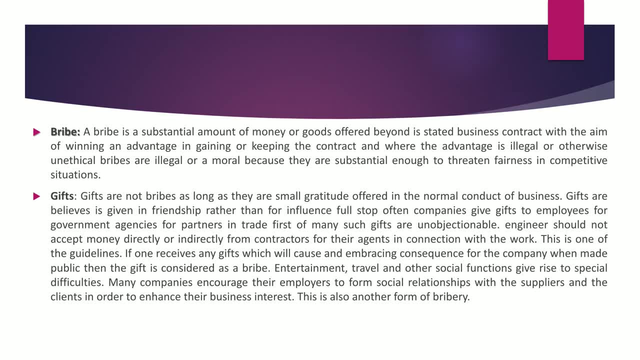 If one receives any gifts which will cause and embrace the consequences of the company when made public, then the gift is considered as a bribe. So entertainment, travel and other social functions give rise to special difficulties. Many companies encourage their employees to form social relationships with the suppliers. 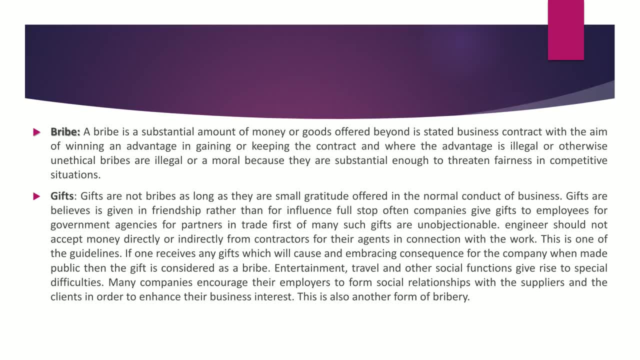 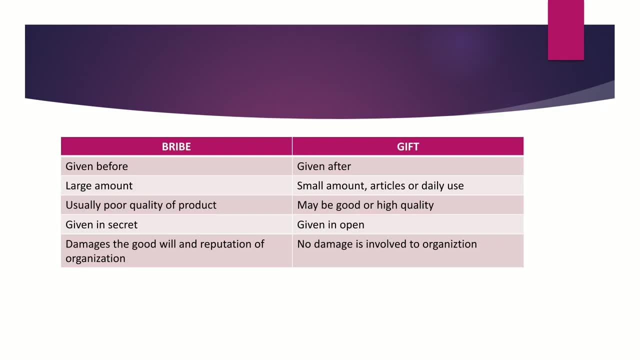 and the clients in order to enhance their business interests. This is also another form of bribery. So what is the difference? So bribe is nothing but given before, and it's a large amount, usually poor quality of product. they will give, And given in secret, and it damages the goodwill and reputation of the organization. 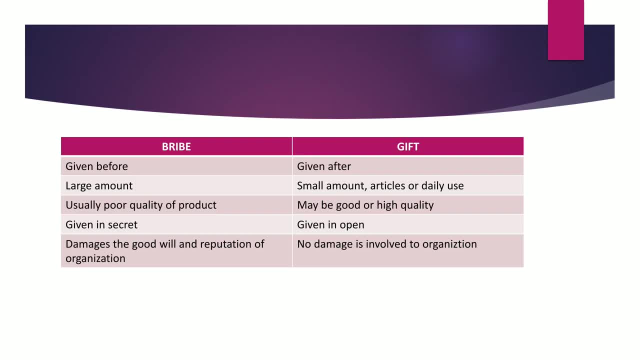 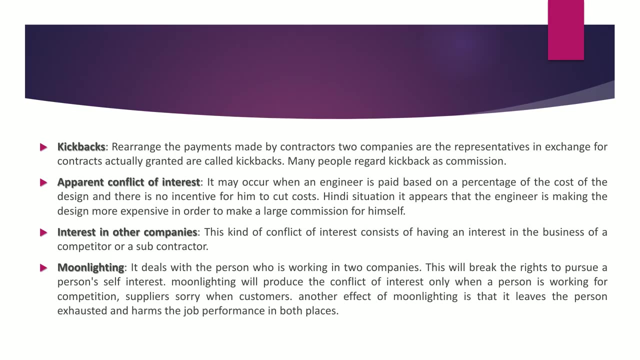 Whereas gift given after the work completed, and it's a small amount, articles or daily use usage things. it may be good or high quality and given in open and no damage is involved to the organization. Next, what is kickbacks? Rearrange? the payments made by contractors to companies are the representative in exchange? 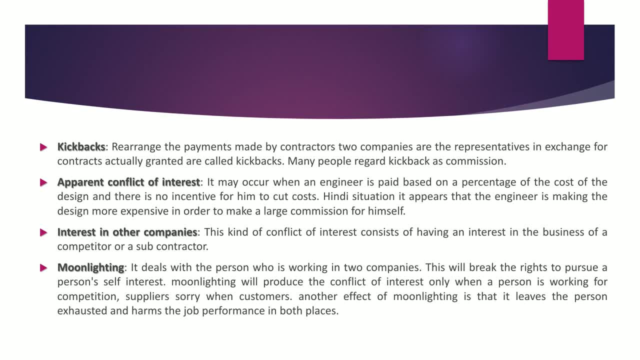 of contracts actually granted are called kickbacks. Many people regard kickback as commission So apparent conflict of interest. It may occur when an engineer is paid based on percentage of the cost of the design and there is no incentive for him to cut costs. 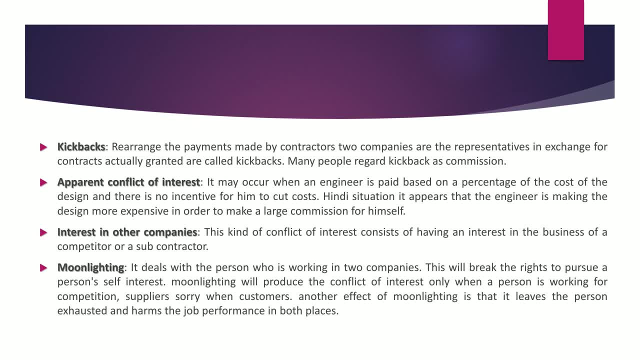 So in this situation, it appears as the engineer is making the design more expensive in order to make large commission for himself. Next is interest in other companies. It's it consists of having an interest in the business of your company. It may occur when an engineer is paid based on percentage of the cost of the design and 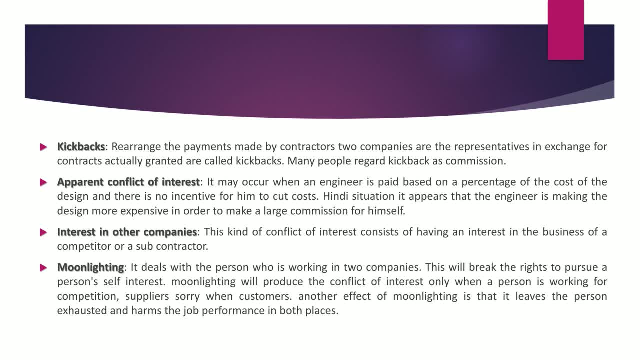 there is no incentive for him to cut costs. So it may occur when an engineer is paid based on percentage of the cost of the design and there is no incentive for him to cut costs. So it may occur when an engineer is paid based on percentage of the cost of the design and 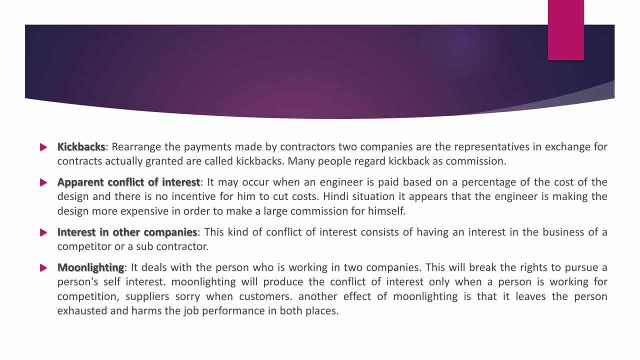 there is no incentive for him to cut costs. Next is Moonlighting. It deals with the person who is working in two companies. So this will break the rights to pursue a person's self-interest, because moonlight will produce the conflict of interest only when a person is working for competition suppliers. 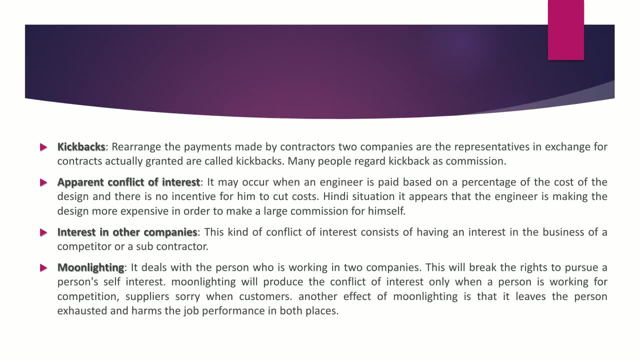 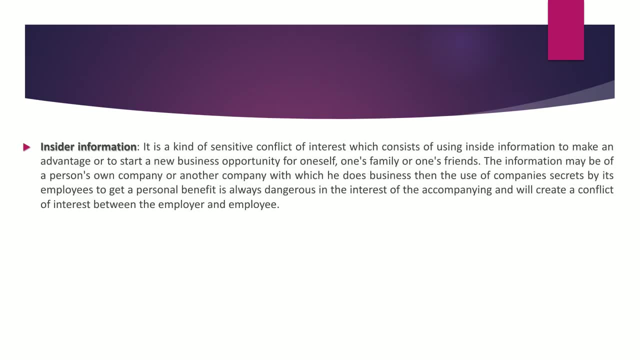 when customers. Another effect of moonlighting is that it leaves the person exhausted and harms the job performance in both the places. What is insider information? It is a kind of sensitive conflict of interest which consists of using inside information to make an advantage or to start a new business opportunity for oneself or one's family or 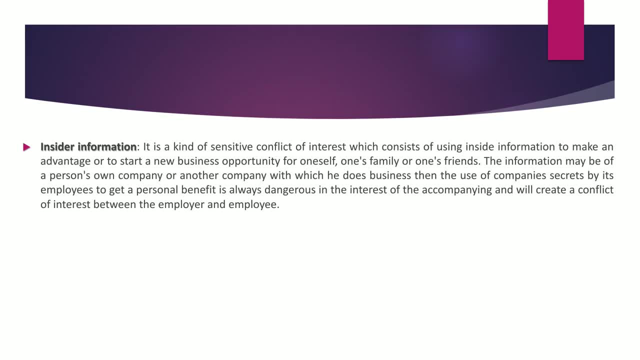 one's friends. The information may be of a person's own company or another company with which he does the business, then the use of company secrets by its employees to get a personal benefit is always dangerous in the interest of the company and will create a conflict of interest. 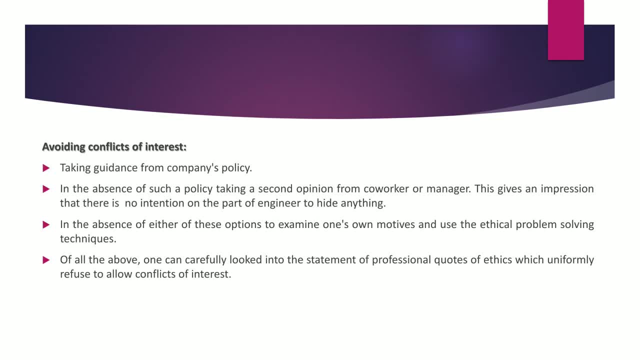 So how to avoid conflicts of interest? Taking guidance from a company's policy- and if it is not there, then taking a second opinion from a co-worker or manager- gives an impression that there is no intention on the part of the engineer to hide anything. 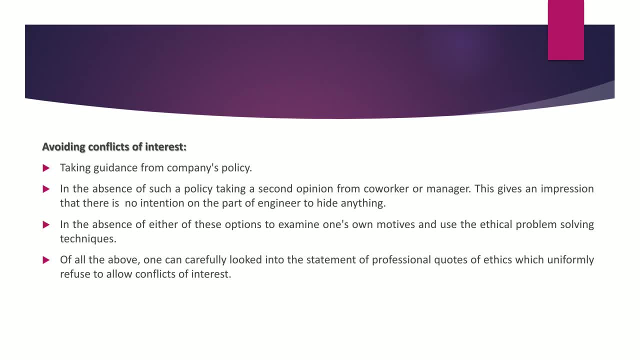 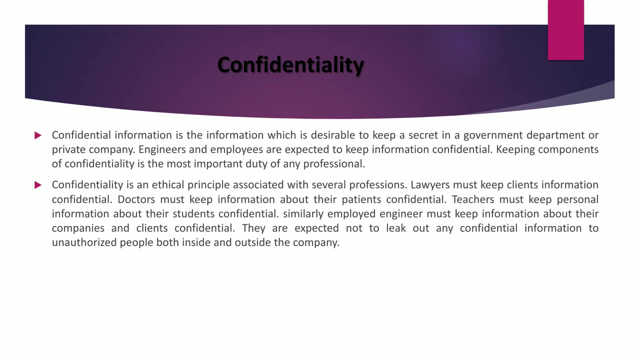 If it is also absent, then examine one's own motives and use the ethical problem solving techniques. And of all the above, one can carefully look into the statement of professional quotes of ethics, which uniformly refuse to allow conflicts of interest. Confidentiality: Confidential information is the information which is desired to keep secret in government. 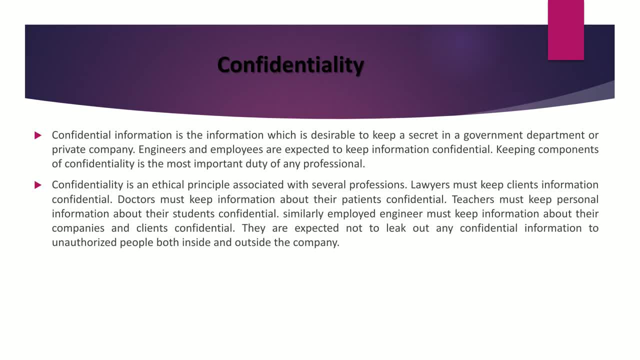 department or private company. Engineers or employees are expected to keep information confidential. Keeping components confidential is the most important duty of a person. Confidentiality is an ethical principle associated with several professions. Lawyers must keep clients' information very confidential, Doctors must keep their patients' information confidential, whereas teachers must keep their. 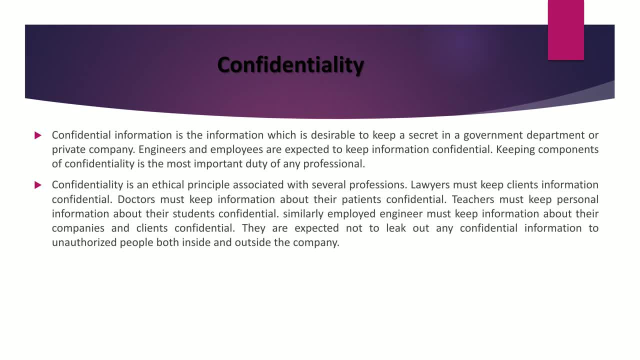 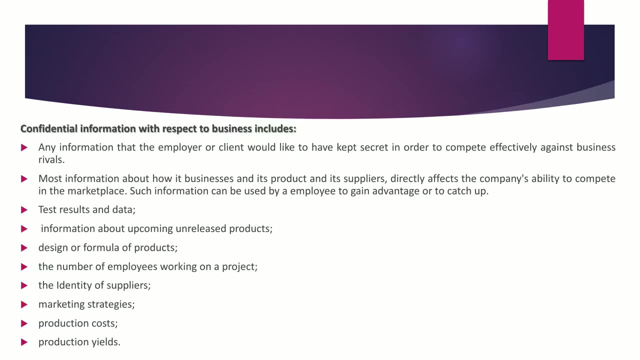 students' information confidential. Similarly, employed engineers must keep information of their companies and clients confidential. They are expected not to leak out any confidential information to unauthorized people, both inside and outside the company. How to avoid conflicts of interest: Confidential information with respect to business includes any information that the 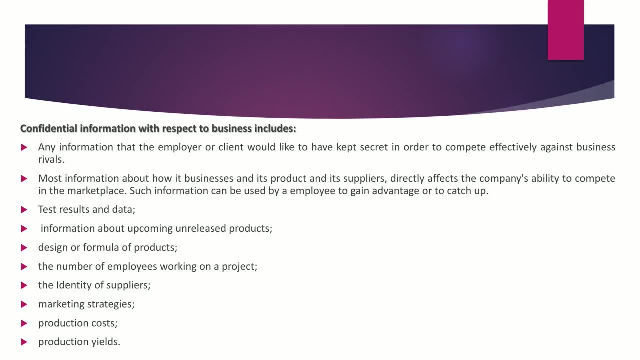 employer or client would like to have kept in secret in order to compete effectively against business rivals. Most information about how it business and its product and its suppliers directly affects the company's ability to compete in the market. Such information can be used by an employee to gain advantage to catch up. 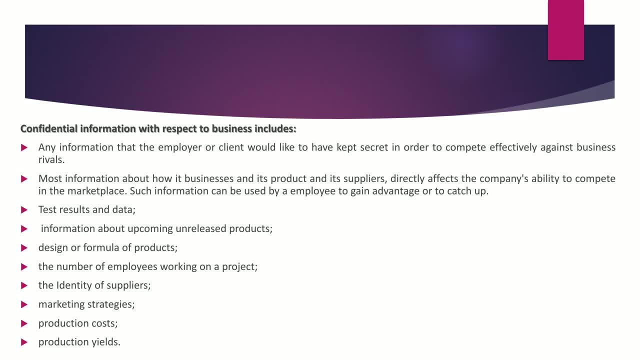 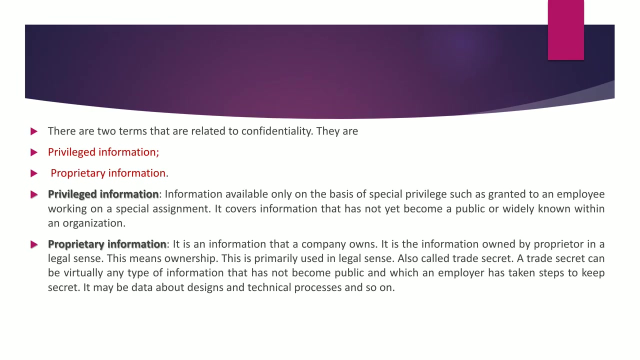 Test results and data. Information about upcoming years. Technology and programming. Product design, Design of the products. Number of employees working in the project, Identity of suppliers, Marketing strategies, Production costs, Production years. Confidential information with respect to Business. Privileged Information and Proprietary Information. Privileged Information and Proprietary Information. 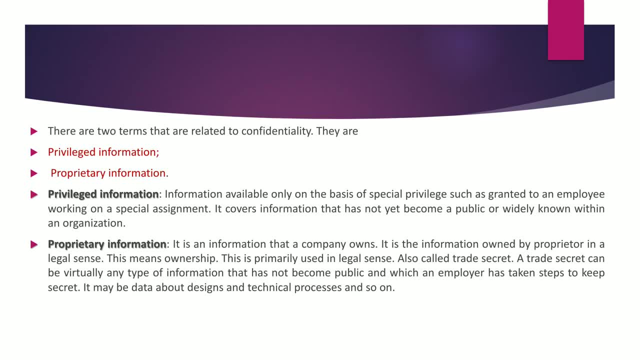 Privileged Information and Proprietary Information. What Is Privileged Information? Privileged Information is an bahasa, indian language- used by the indian government to promote This information only based, available only on the basis of special privilege, such as granted to employees working on a special assignment. 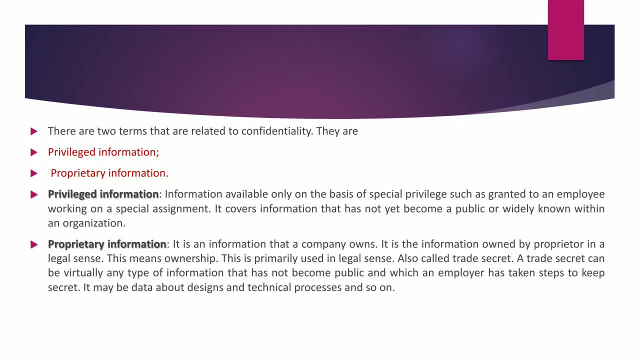 So it covers information that has not yet become a public or widely known within an organization itself. So proprietor information is that a company owns. It is information owned by a proprietor. in a legal sense, This means ownership. This is primarily used in legal sense, also called as trade secret. 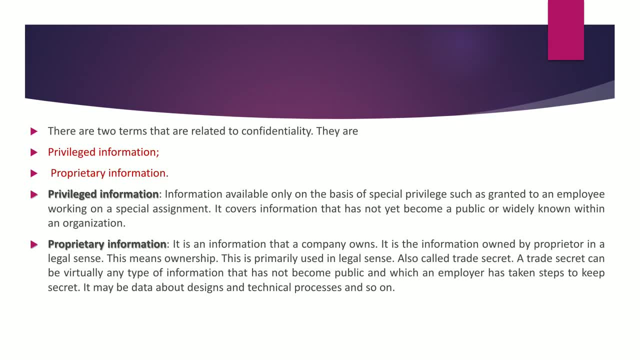 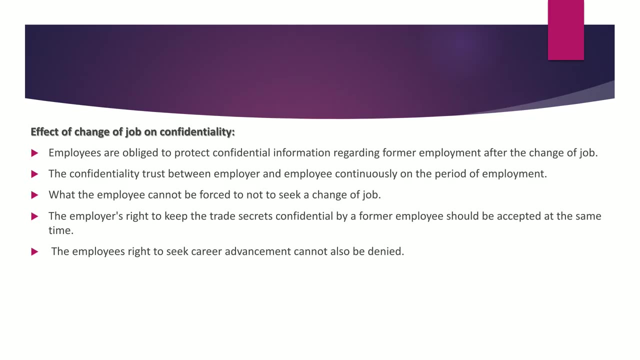 A trade secret can be virtually any type of information that has not become public and which an employer has taken steps to keep secret. So it may be data about designs, technical processes and so on. So effect of change of job on confidentiality If you change your job from one company to another. 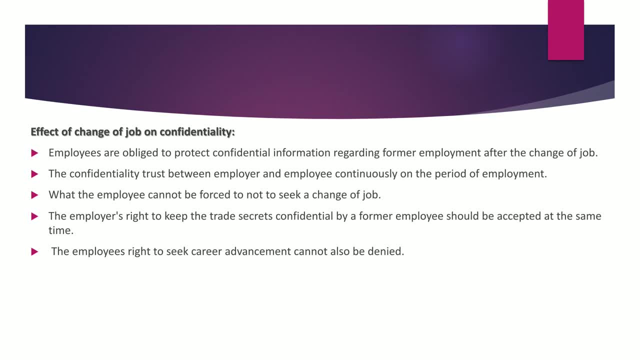 So what actually? it affects into the confidentiality of previous company. So employees are obliged to protect confidential information Regarding former employment after the change of the job. The confidentiality trust between employer and employee continuously on the period of employment, What the employee cannot force to not to seek a change of job. 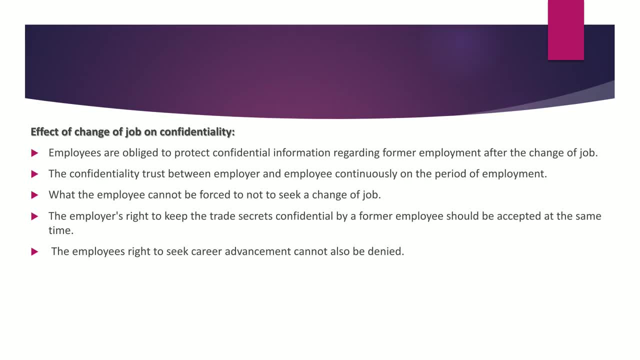 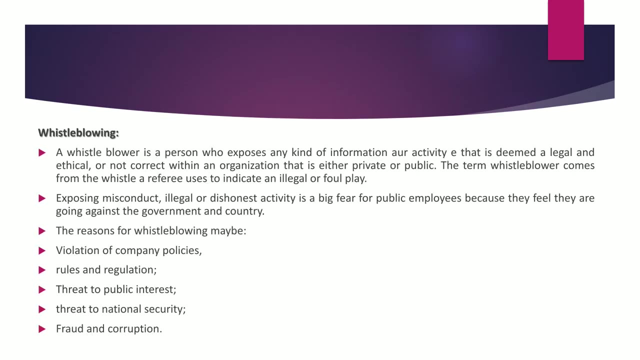 Next, The employer's right to keep the trade secrets confidential by a former employee should be accepted at the same time, And employer's right to seek career advancement cannot also be denied. So last topic is whistle blowing. A whistle blower is a person who exposes any kind of information or activity that is deemed a legal and ethical or not correct within an organization that is either private or public. 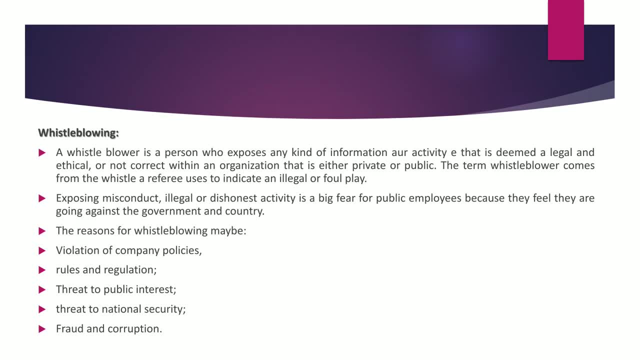 The term whistle blower comes from the whistle a referee uses to indicate an illegal or foul play. So exposing misconduct or dishonest activity is a big fear for public employees. The reason for this is the victims are actually the whistle blowers, because they feel they are going against the government and a country. 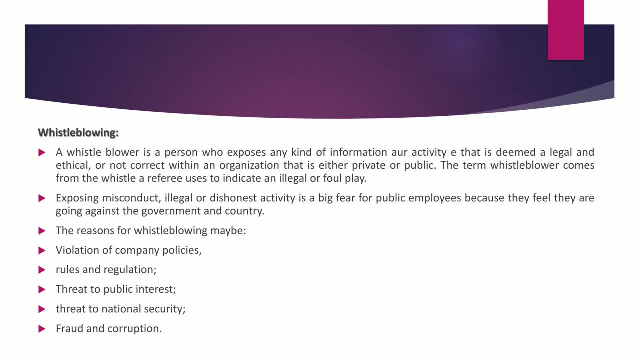 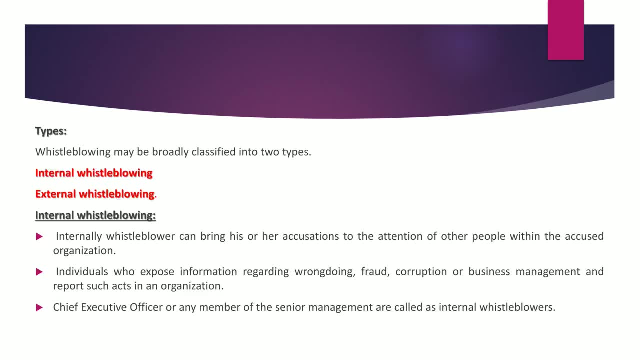 So the reasons may be violation of company policies, rules and regulations, threat to public interest, threat to national security, fraud and corruption. There are two types of whistle blowing. Those are internal whistle blowing and external. So what is actually internal whistle blowing? 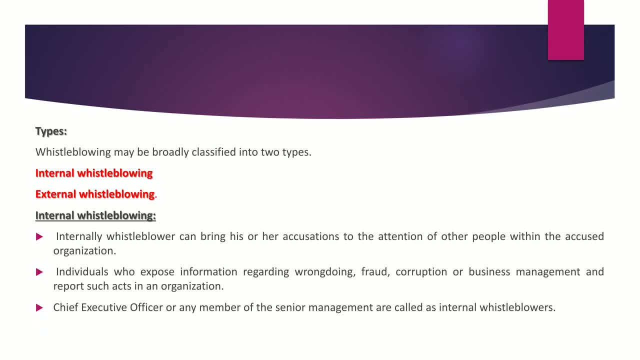 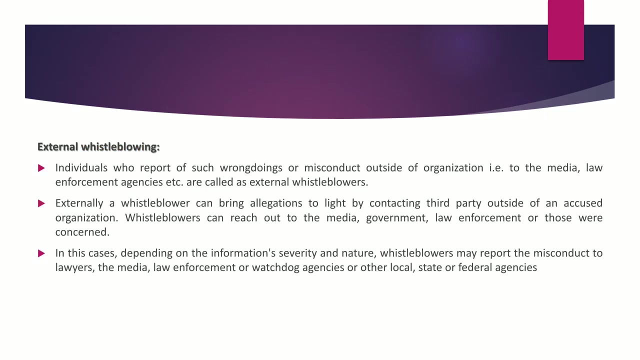 Internally, a whistle blower can bring his or her acquisition to the attention of other people within the accused organization. individuals who expose information regarding wrongdoing, fraud, corruption or business management and report such acts in an organization- usually the chief executive officers and senior management- are called internal whistleblowers, whereas external whistleblowing is individuals who report. 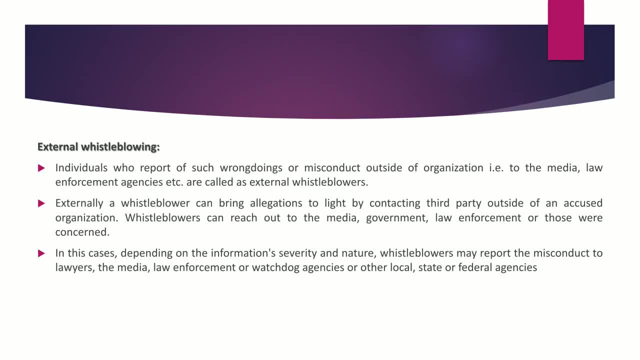 of such wrongdoings or misconduct outside of organization, that is, to the media and law enforcement agencies etc. are called external whistleblowers. externally, a whistleblower can bring allegations to light by contracting third party. outside of an accused organization. whistleblowers can reach out to the media, government, law enforcement or those were concerned.